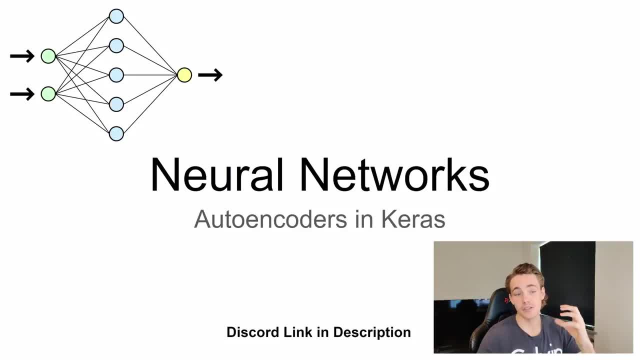 can set up auto encoders and carriers, because these auto encoders is actually really useful in modern deep learning and neural networks applications and projects. But first of all, remember to join the discord server. I'll link to it down in the description. here You can come. 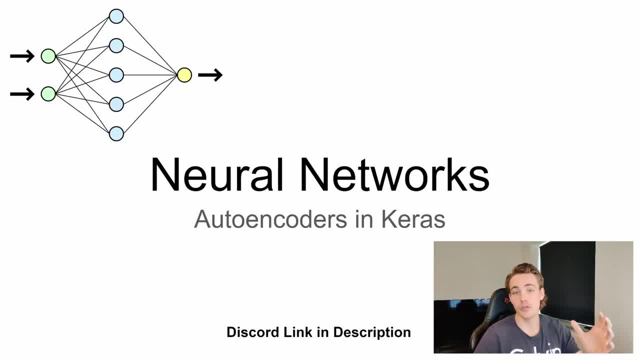 join the channel, share it with your computer vision, deep learning, AI and so on. You can also become a member of the channel if you want to support the channel, with a small monthly fee. Everything will go to create more and better quality content here on the channel. Also, if 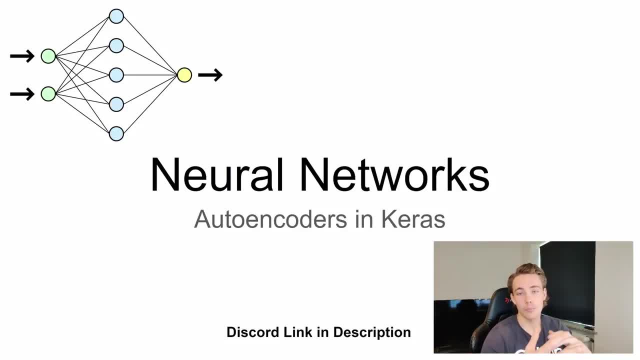 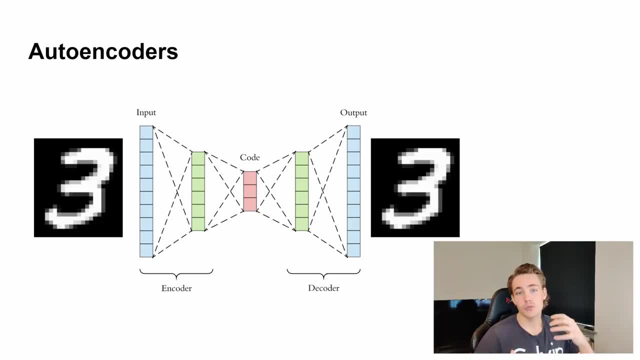 you're a member of the channel, you can also get some personal help with your own problem or on your own projects. if you have some problems, I can help you out if you're a member. so thank you guys. So first of all, here we're just shortly going to talk about what auto encoders are. I've 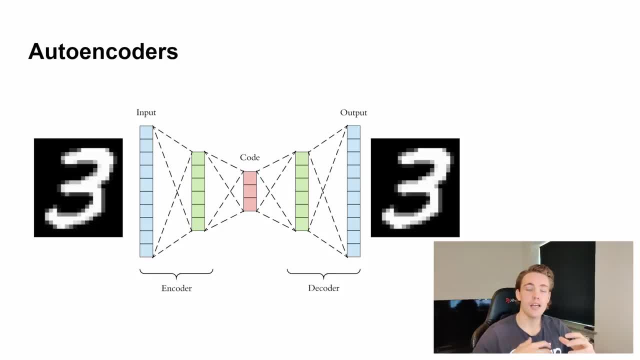 already made a video where we went more in depth with auto encoders and then we did the code in PyTorch. but in this video here we're just going to shortly cover what auto encoders are and then we're going into carriers to actually see how we can implement it in carriers, as we're done. 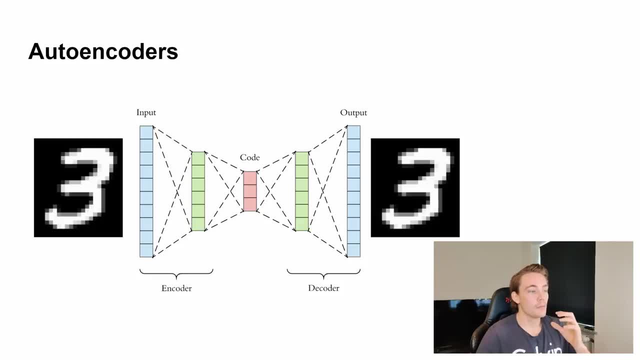 throughout the whole tutorial here with TensorFlow and carriers, But auto encoders here you can actually like be used for compromising data and so on, as we're going to do in the code example in this video. So we'll say that we're taking the endless data set with these handwritten digits. 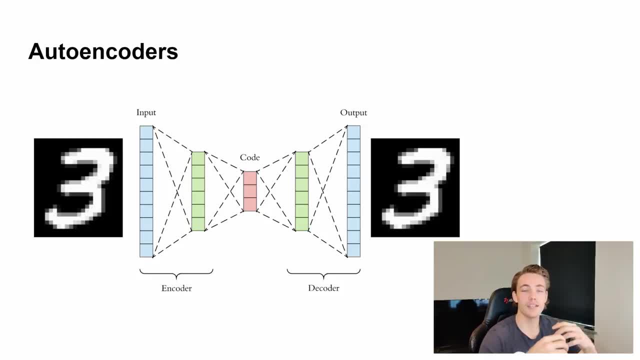 then we can actually like pass it through these auto encoders and then we'll end up with this code vector, as we can see here in the red or like the orange color. So we're actually just downscaled all like the information about our images, So we can take our input image, which is: 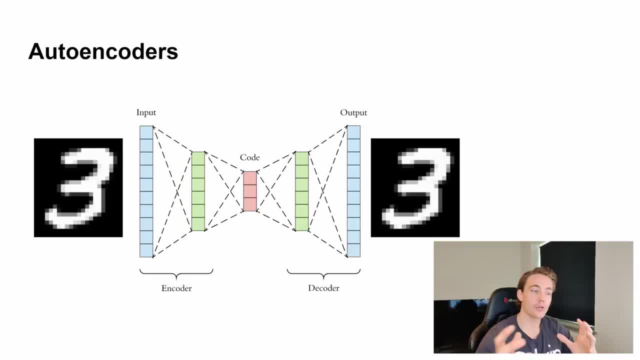 free here to the left. then we just pass it through our neural network, layer by layer, and then we get this code vector, which will just be different kind of features, Features that describing the image that we fed through our encoder side. So we both have an encoder side. 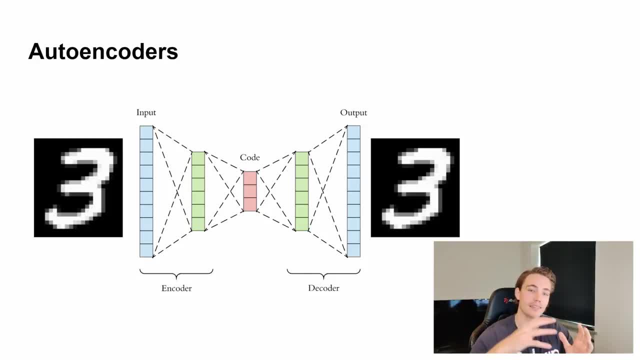 we have our code vector and then, after we have our code vector, we can actually decode that code vector again. so we like reconstruct our input. So we have the input, we just pass it through the neural network. then we, then we compromise the information and the features in our image down. 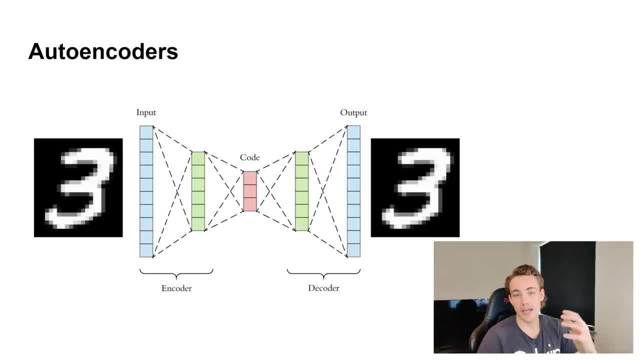 to a vector with an arbitrary number of values. You can use eight values depending on like the complexity in your image, and then you can just decode your image again and reconstruct it, as we can see here on the right hand side. So we're now straight into the fun. 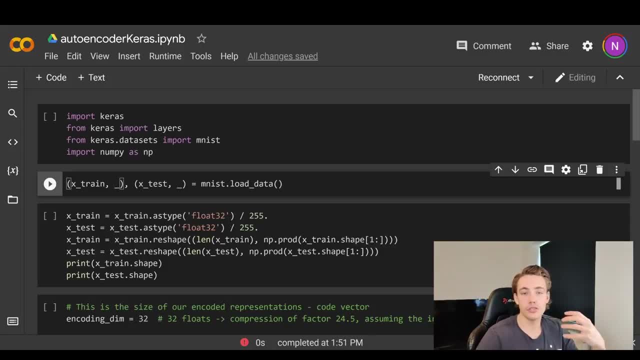 part here in the code. So we're using Google Colab here and also the GPU in Google Colab to actually train our neural networks, as we've done in all the other videos throughout this neural networks and deep learning tutorial. So first of all here we're just going to import the modules. 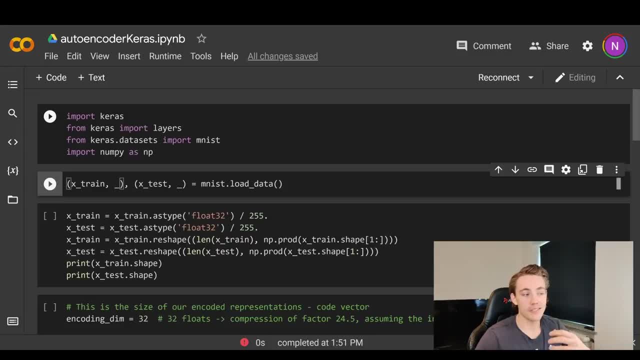 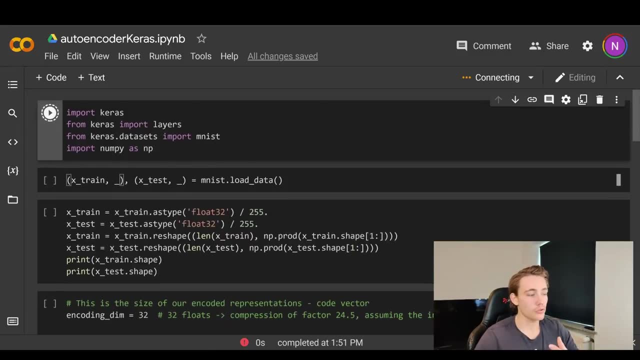 that we need. So we're going to use Keras and we're also going to use the MNIST data sets. that is already implemented in Keras, and also we're going to use the MNIST data sets. that is already implemented in Keras. So we're just going to run this block of code so we'll import the modules. 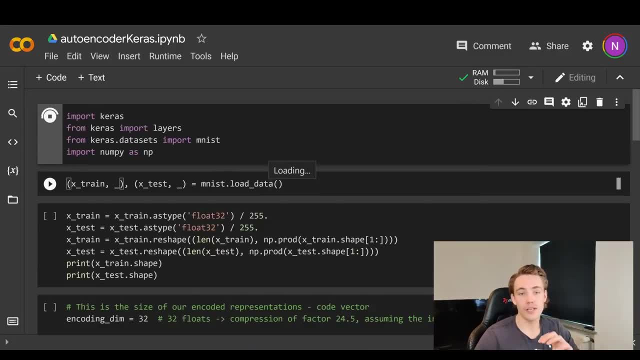 then we just go down here to the next block of code where we're just going to load in the MNIST data set. We just call MNIST here because we imported it up here from Kerasdatasets- and then we're just going to call load data and then we can actually just store our data in our training set. 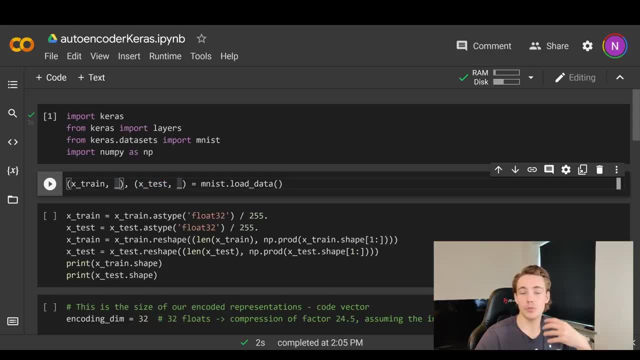 and also in our test set. We don't really care about the labels here because we're just using an also encoder, so we don't need labels for those images. We just want to have an input image. then we can actually like compromise that data so we actually like have less features. so instead of 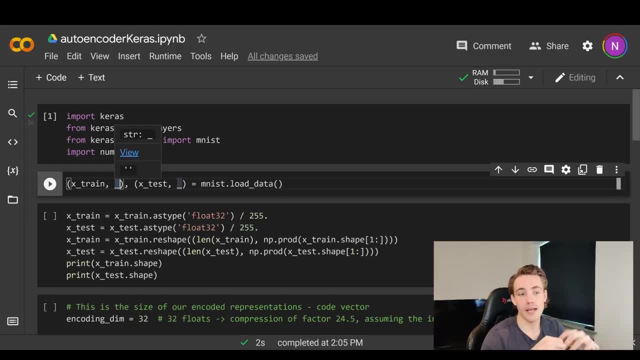 we have an image that is maybe like 28 by 28 in the dimensions, then we will have like 700, 784 values representing or like describing that image. we can actually like compromise that down to only like five, eight values describing the whole image and then we can reconstruct it with a really low loss. 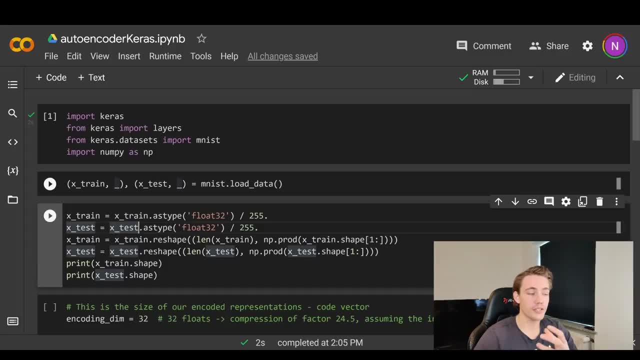 So here we're just going to run the plug code and we will just store our training set and also our test set. So we're training our neural network on the training set And then we're going to go ahead and and then we're doing the tests on the test set. so the test images is actually like new images. 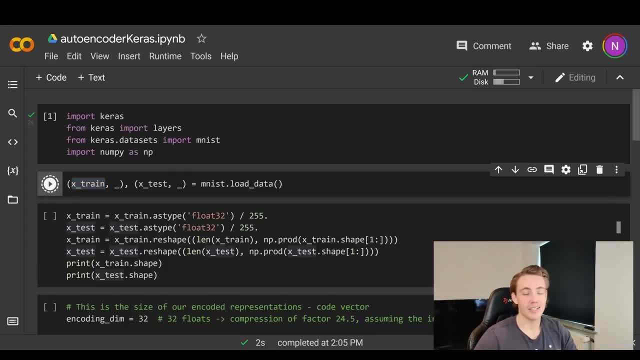 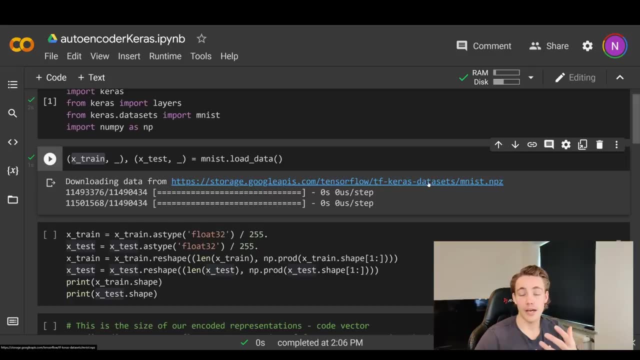 that the neural network hasn't trained on before, So we get a general model that is not overfitting. So here we're just going to download the data set. We can see that it just downloads it from the Keras data sets and we can also see here that it's now finished. Then we need to pre-process. 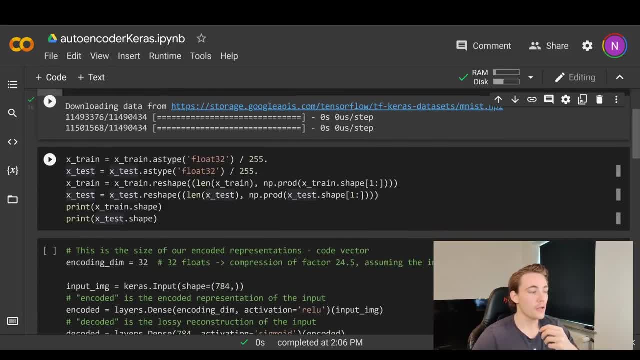 our data set before we can actually like pass it through our neural network. So first of all we're both going to do the same thing for training set and the test set. So first of all we're just normalizing our images. so all the pixel values, so these are the intensities that we're just 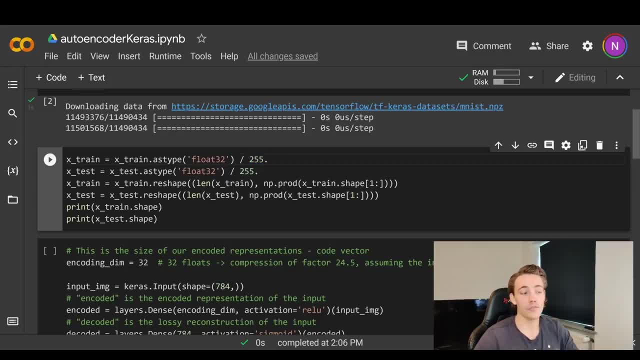 dividing by 255.. So we're normalizing it. so all the values in our image is actually like between zero and one, which is just good when we are talking about neural networks and how to learn- learn under the hood. We're going to do the exact same thing for our test set and then down here we. 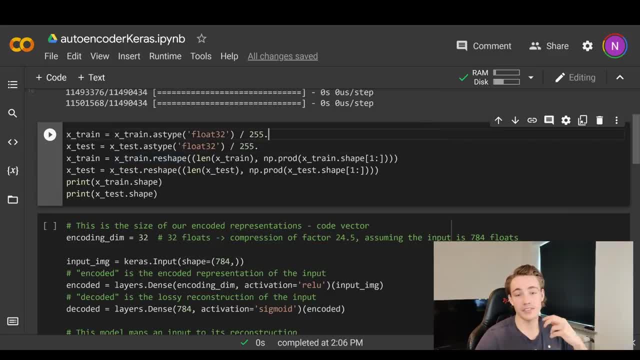 need to reshape it, because we're just going to use and like a standard artificial neural network where we just have these different kind of like nodes or neurons in our network. So we're not going to do that. So we're just going to do the same thing for our test set and then down here. 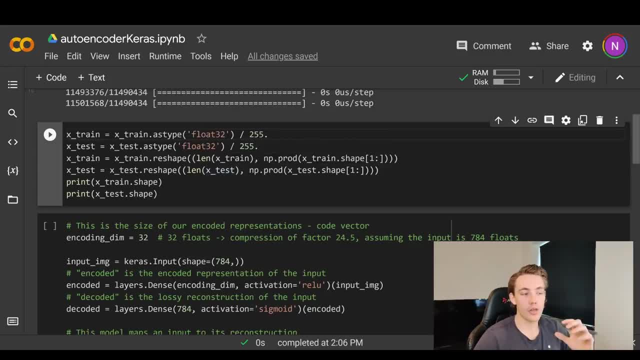 we're not going to use convolutional neural networks in this video, but I'm going to create another video with autoencoders, where we're using convolutional neural networks to actually like do autoencoders with images. But in this video here we're just going to flatten our, our images. 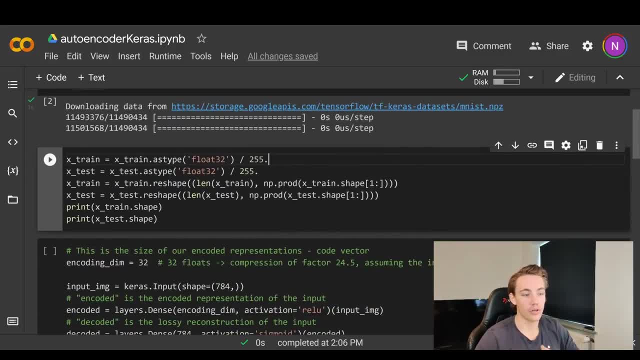 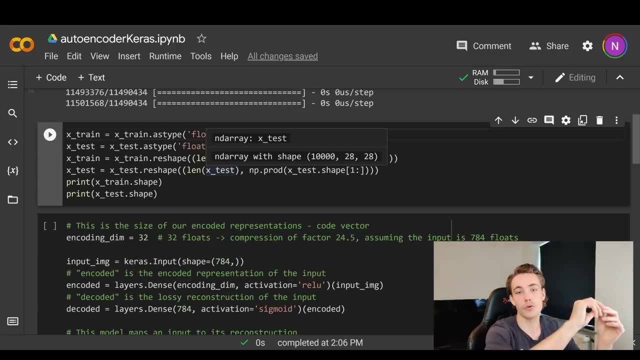 so instead we have like a 28 by 28 or or the dimensions of the MNIST data set. Then we're just going to have one vector where just all the values are stored, like: so take the first row and then we just append the second row after that one. so we just have one vector with the size of 700. 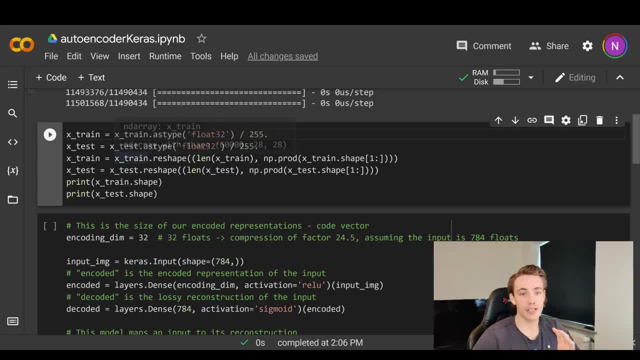 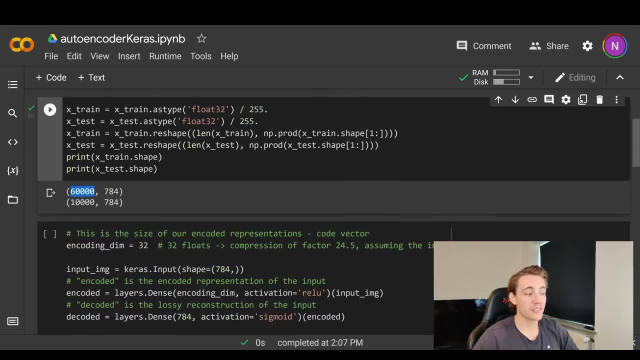 and 84, as we can see down here. So we actually we just flatten our images in our test set and our training set and then we're just going to print the shape here. So when I run this blog code, we can see that we now have 60 000 images from the image data set in our training set, and this is 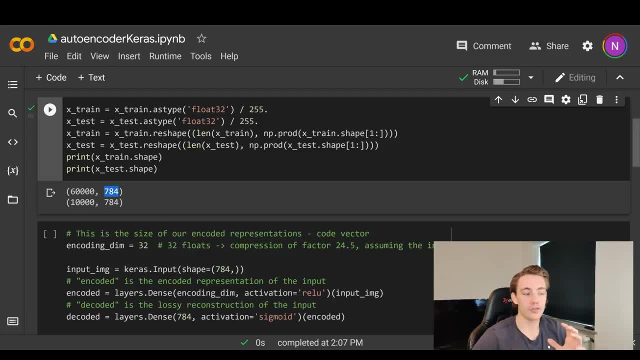 the dimensions or the shape. so we'll just have one vector with 784 values in that, and then we have 60 000 of those vectors with this dimension. We're going to have the exact same thing for our test set, but in our test set we'll only have ten thousand values, and then we're going to have 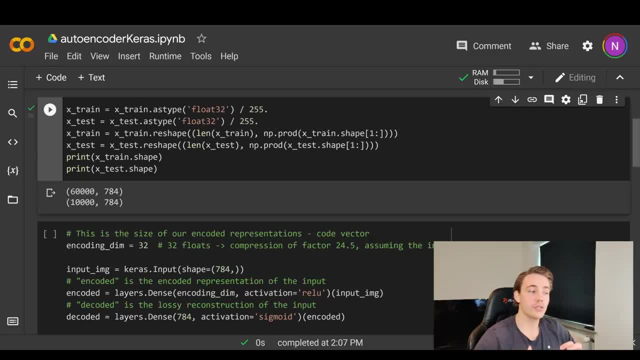 60 000 images instead of 60 000 images. So when we're going to train our neural network, we will actually pass 60 000 vectors of this dimension through our neural network for each epoch that we're actually training our neural network on. So now we have set up our training set here we 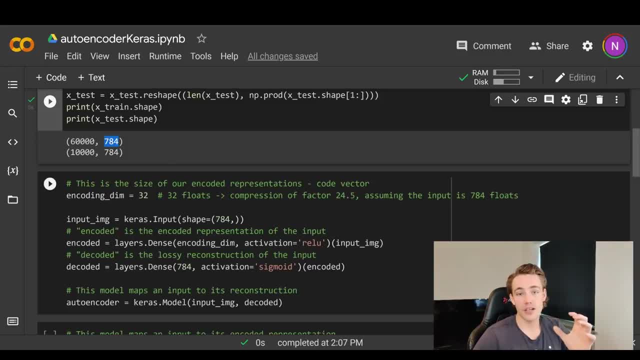 can actually start implementing the autoencoder. So again, as we know from the slides, we need both an encoder side, we need a code vector representing all, or like storing all features from our input image, and then we're going to have our decoder side that tries to map. 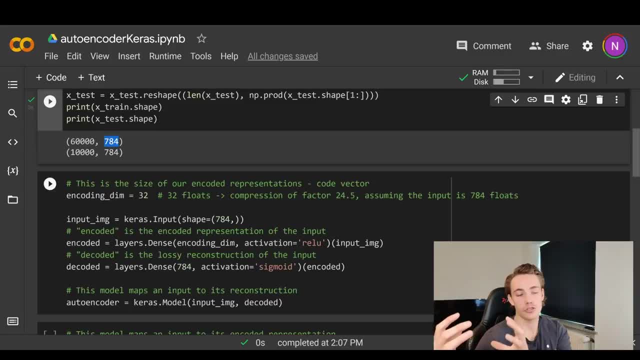 from the code vector or feature vector back to the reconstructed input image. So here we're just going to choose the dimensions from our encoding, or like the size of our code vector, as we can see here. so we're just going to choose 32. here we can also try 16 and 8, because this is actually like a. 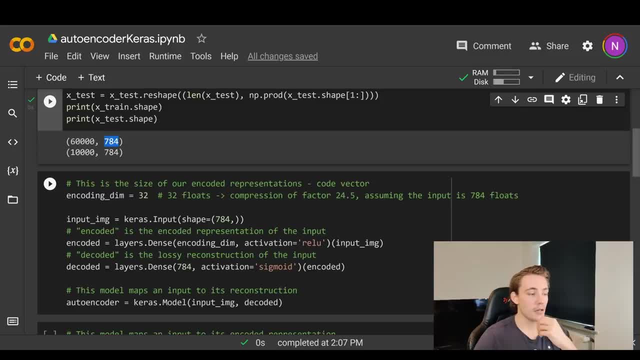 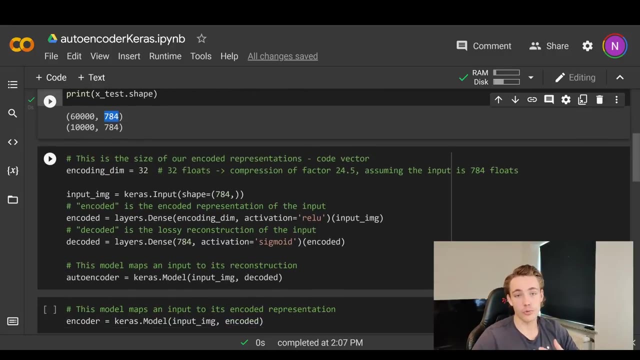 really simple image when we're only using the MNIST data set. but if you have more complex images, you can try with 32, 64 and so on. like you just choose an arbitrary number in the encoding dimensions or the size of our code vector, so here we can see that we have 32 floats, that we're storing all the values from our images. 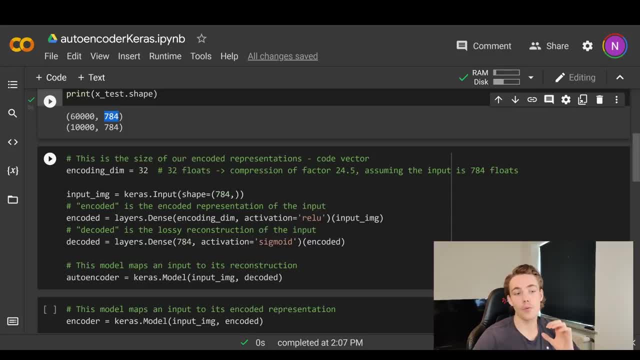 in. so this is actually a compression of a factor of 24.5 if we assume that that the input is actually 784 floats. so this is a really significant compression factor when we're actually like doing this and, as we're going to see, we will not lose that much information, or like that. 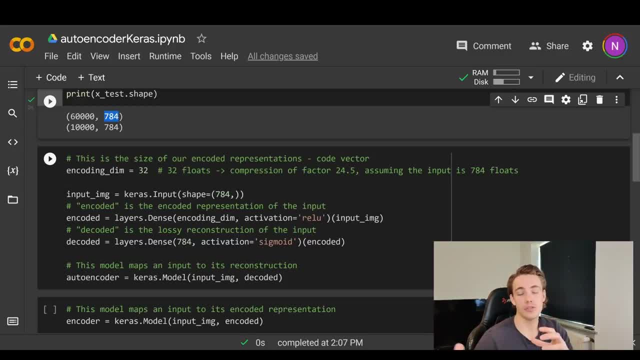 much information in our in our actually reconstructed image. So here we're just going to use the input image, we're going to use carriersinput, so here we're actually just setting our input layer of our neural network and the shape here will actually just be 784. so this is. 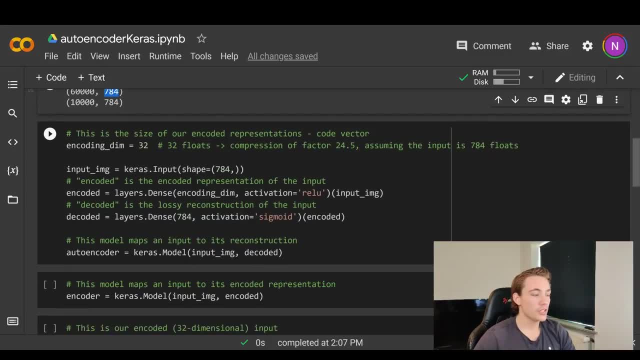 just one vector representing one image that is flattened. so here we can have our encoded encoder. here is the encoder representation of the input. so this will just be the end after our actual like, after actually like, encode aside. so in this example, here we just have one encoder layer. 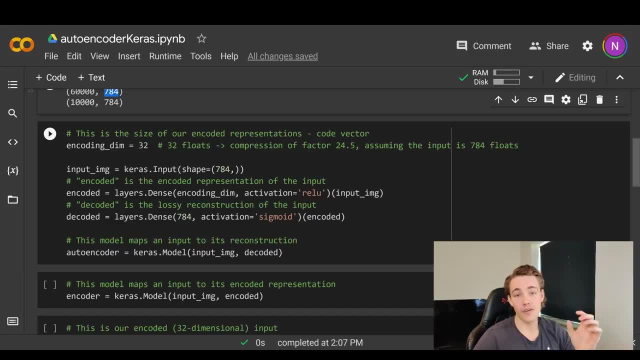 and one decode layer and then we have our our code vector. so i'm very sure as well how we can actually create a deep auto encoder where we actually have multiple hidden layers inside of our model. but, as we're going to see, if we just have one encode layer, one decode layer and one code vector, we can actually get really nice results. 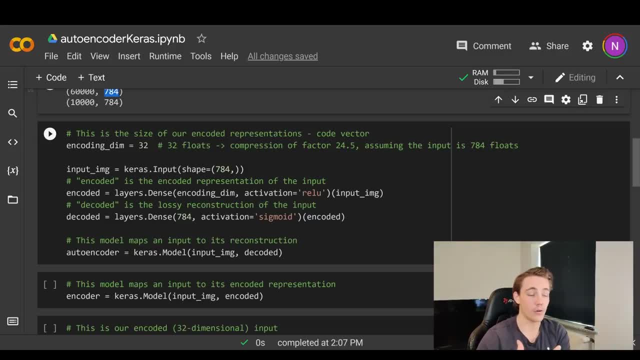 without, like even having that many neurons in our neural network and and also a really, really or like the simplest neural network that is even possible. so here we're just going to set our encode here equal to layers. so we're just going to take a dense layer because we're using artificial 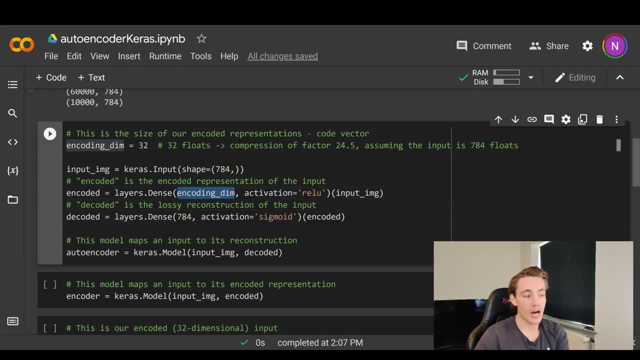 neural networks. then we set the encoding dimensions here, which is the output of our dense layer. so the number of neurons in our output layer, or like in our, in our, in this encode layer. so that's what this will be, the dimensions of our covector. we set the activation function, we 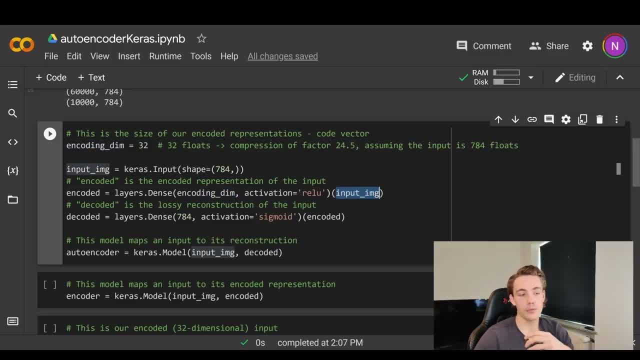 use value. and then we just- i could like put it together with this input image, uh, input image layer, as we can see up here. so here we're actually just creating a sequential model or actually constructing a neural network. then we also need our decode layer after our. 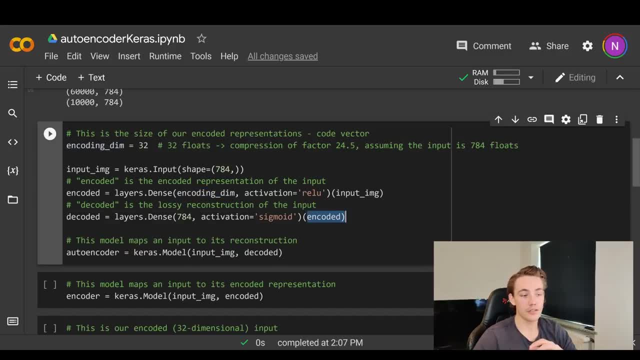 encode vector. and then, here again, we're just going to pass here through the encode layers. after the encode layer, we're just going to have the decode layer where the output, um, where the size of the output is 784, because we actually want to reconstruct our image, so so our input is 784. 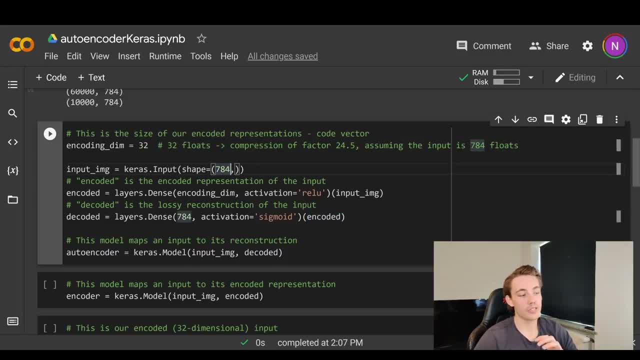 then we have one layer with 32 neurons and then we just have our output layer with 784 neurons that is trying to represent, or like reconstruct, our image from the input. then we're going to combine it. so this model here mapped the input to its reconstruction, so we're going to create the whole. 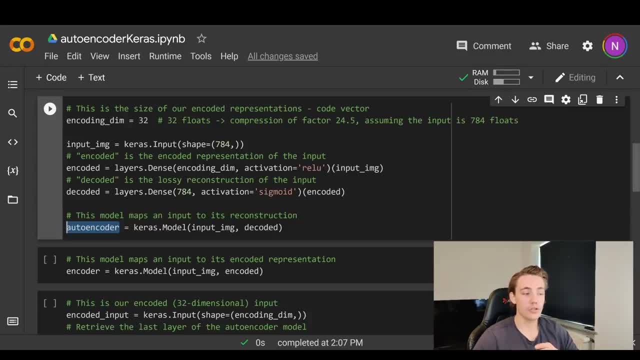 other auto encoder here. we just set it equal to carriersmodel, so now we're actually just creating a model from carriers that we can then compile and train on with our data set. we just pass in the input image here and also the decode here, because we have put it all together here in. 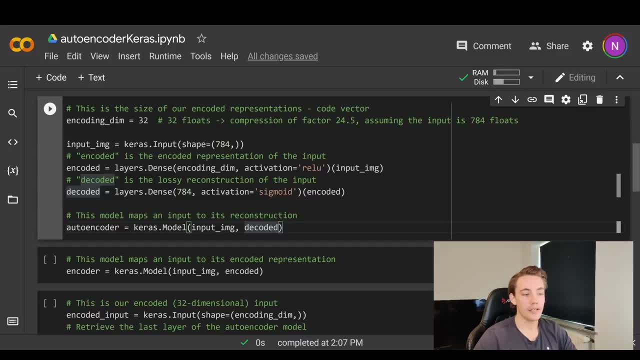 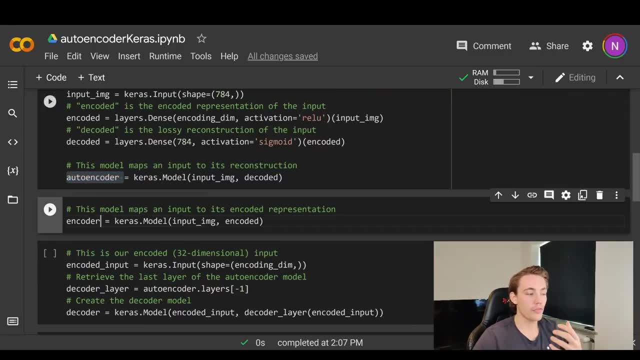 the sequential model by having this like input here and then also the encoder here at the end of our layer. so now we have a whole auto encoder here. we can also create both an encoder and a also a decoder, as we're going to see. but now i'm just going to run this block of code so we actually 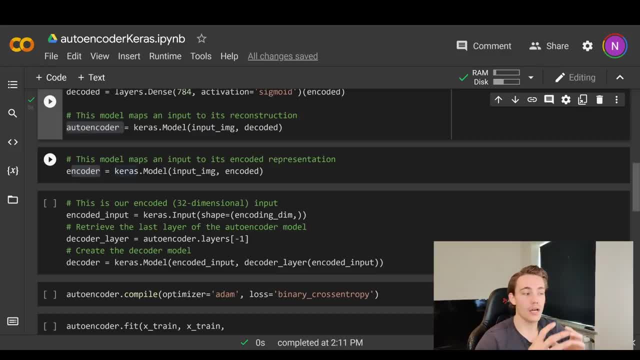 create an awesome encoder, but when we're going to show what the encoder actually does and what the decoder does, we're just going to divide those things in as well. so this is the whole auto encoder, but we're also going to just create an encoder, so like the encoder side, and then we're also going to 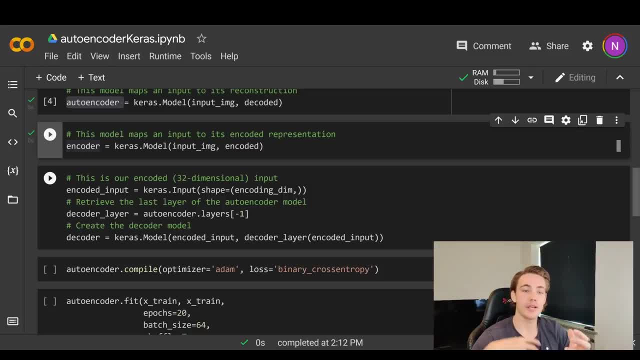 to create a decoder side here so we can separate them in and then we can actually see what is going on in the encode layers and also in the decode layers, uh, when we're working with our third two-dimensional code vector. so here we're just going to set our input here as our encoded input. 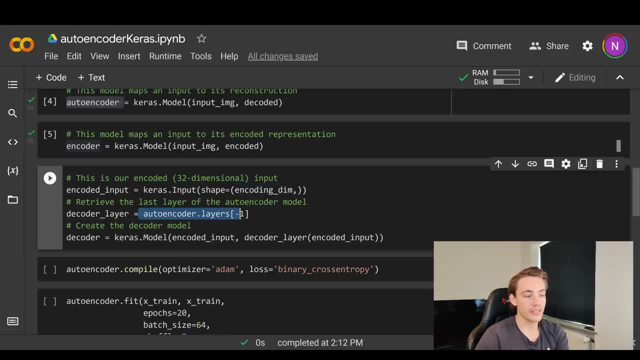 which is the dimensions of our code vector, and then we're just going to take the last layer here of our auto encoder, which will actually be the output of our decode layer, and then we can set up the decoder here, where we just pass in the encoded input and also the decoded layer here. 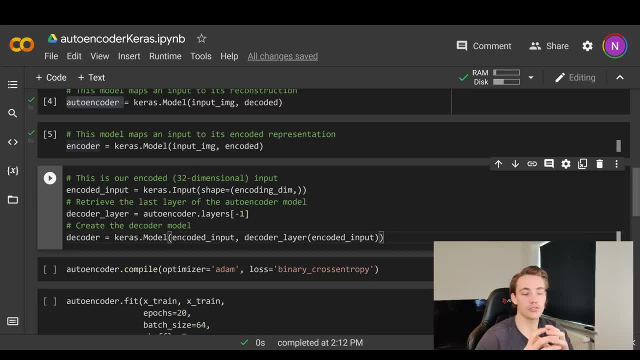 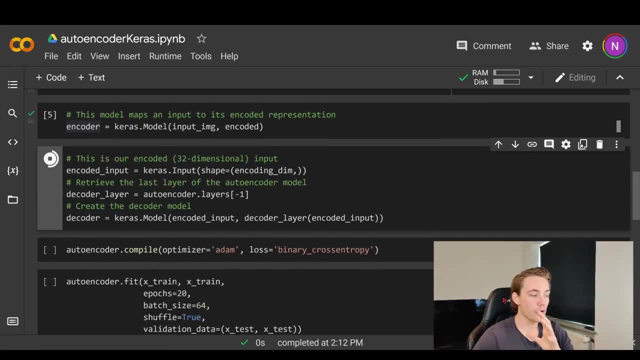 for the encoded input. so this is just how we can reconstruct our image so we can see what is going on on the decoder side later on. so we're going to run this block code. we have now created both our encoder, our decoder and the total combined auto encoder up here. then we can compile our auto encoder and then train it on our data set. 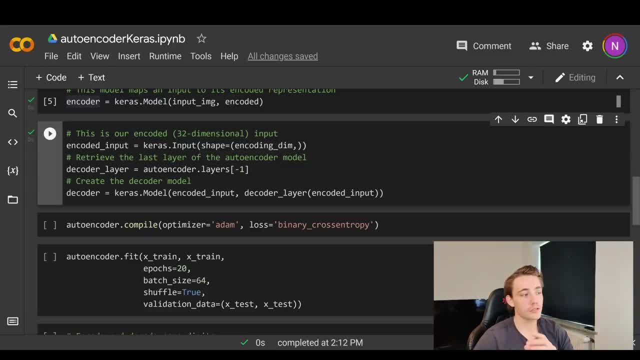 and then we can go in and take individual, individual layers with the encoder and the decoder and also the code vector so we can see exactly what is going on in our auto encoder. so now we're just going to compile our neural network with the atom optimizer and we're going 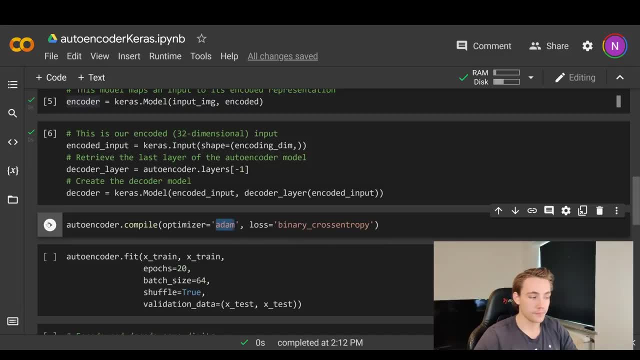 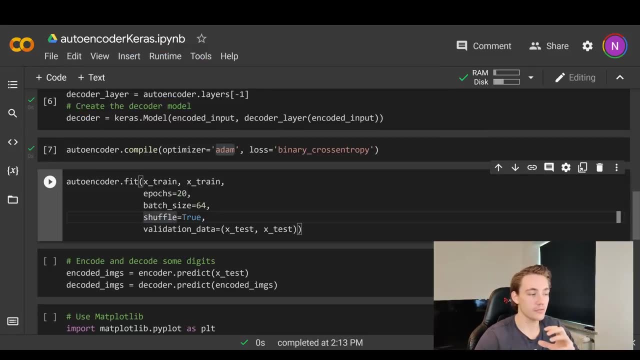 to use binary cross entropy as the last function. so we're going to compile a model, then we're going to train it with this fit function. as we know, throughout this tutorial with keras and tensorflow, we pass in the training training images here. as we can see, here we need to pass it in twice because we're just using auto encoders. 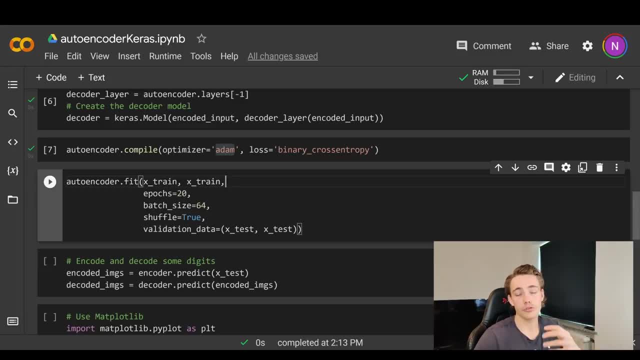 and we're not really having labels or we don't need labels to train our auto encoders. then we're going to specify the number of epochs that we want to train up for. so in this example we're just going to go with 20 and also the bat size of 64. we want to shuffle the data set every time we 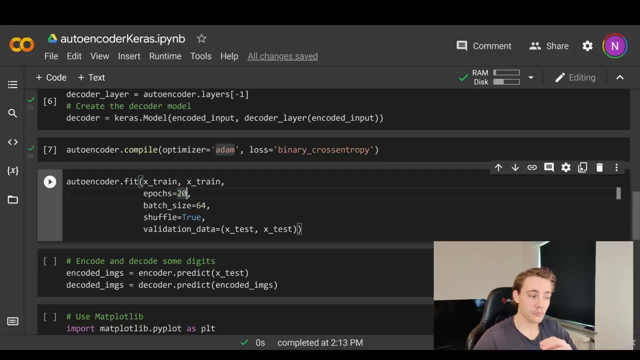 truck through a new epoch. um. so we actually get some random- like some random- order in our training process. our validation set will just be our test set in this example here. so we're just validating on our test set. so now we're going to run this blog code. we will actually start. 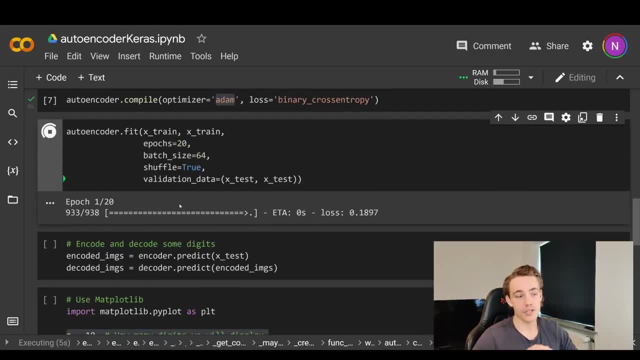 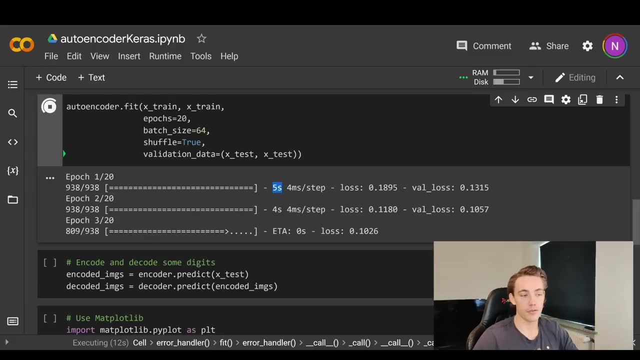 the training process of our neural network and i've set the, the hardware accelerator, right here to the gpu so we would actually like train on the gpu so it runs uh way faster. we can see like each epoch takes around 5 seconds. 4 seconds here after i load in all the images. 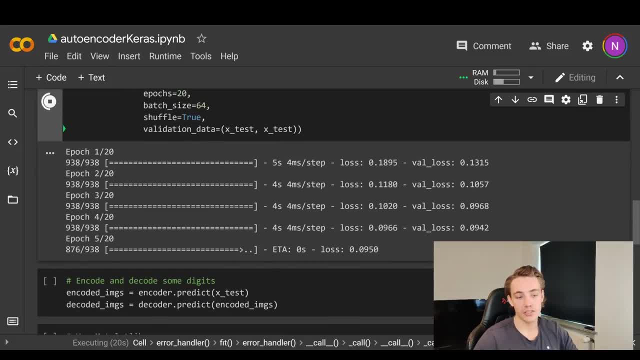 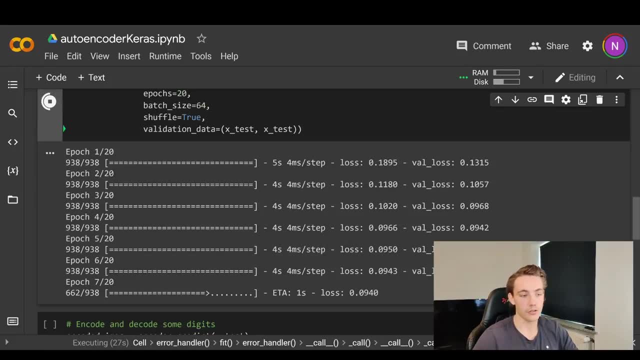 cache. we can then see the loss and also the validation loss here, and it should decrease over the number of epochs until it has converged to some, to some certain value. so here we start with a loss of 0.19 and a validation loss of 0.13. so the reason this is lower is actually like: 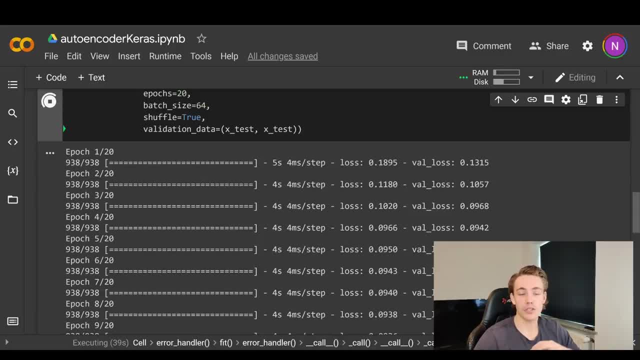 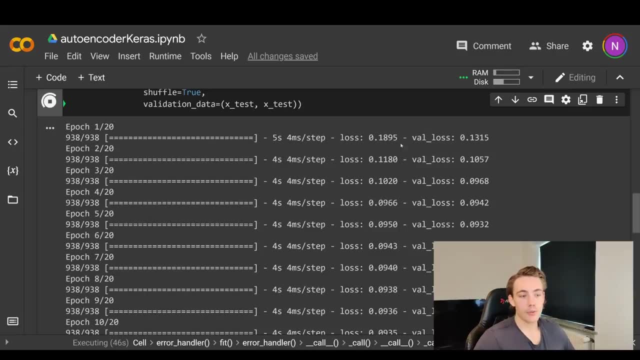 because for each of the batches it is actually calculating the loss, but the validation loss is is first calculated after all the batches, or like at the end of the epoch. so now here we can see that the loss is actually like decreasing, both for the loss and also for the validation. 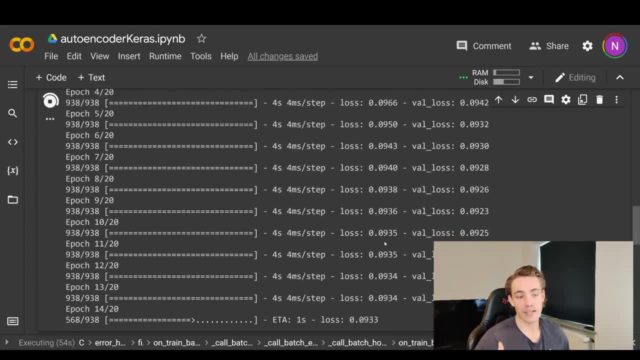 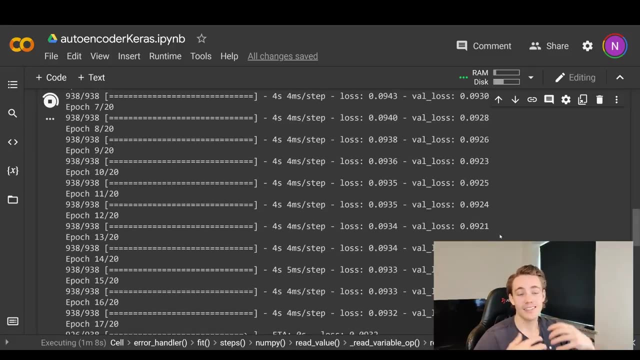 loss and down here after like 10 epochs, we have actually like already already converged to to a loss of 0.09 and also 0.09 here in the validation loss. so actually i have a model that is pretty good both- both at generalizing and doing reconstruction of images- that it hasn't seen. 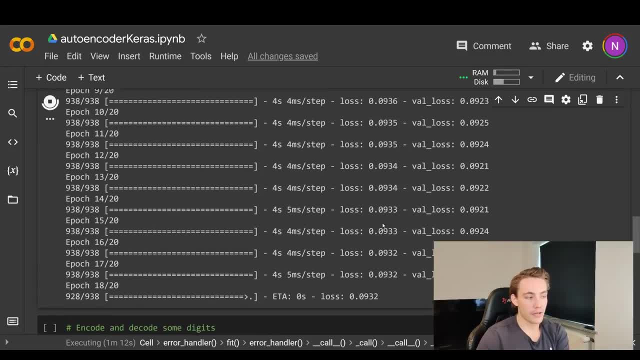 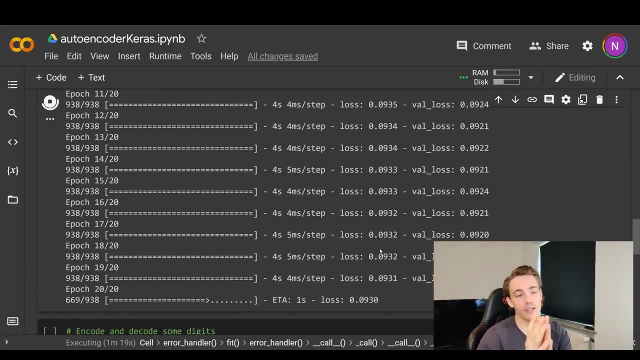 or like it hasn't trained on before. we see here: it doesn't get better from like epoch 10 to epoch 20. so this will be the end results when we're only using one encode layer, one decode layer, And then we have 32 floating values in our code vector. that is actually. 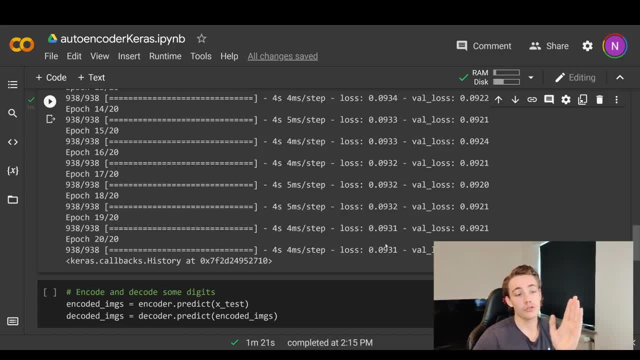 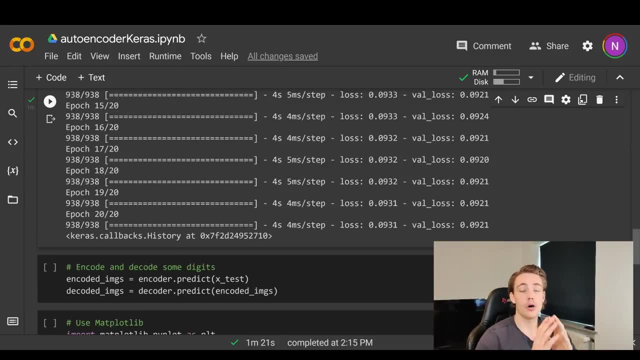 representing the whole image, And then we can use those 32 values to reconstruct our whole image Um later on again, with a loss of around 9%. So we get nine, nine 9% loss, but we can also store our image in in in way. 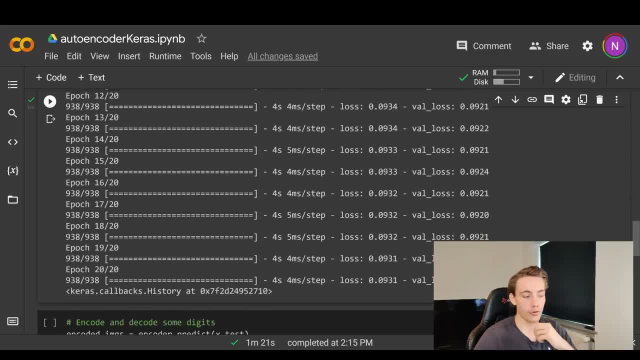 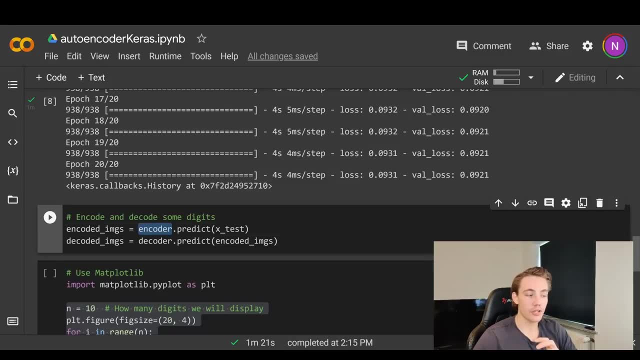 like with an opto factory like um of 24.5 times. So now we're just going to encode some images. We're going to call predict. So we're going to use our encoder that we've trained, and also the decoder. 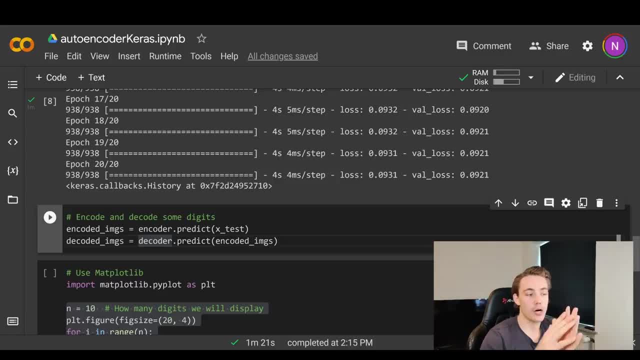 So we trained the whole auto encoder together. but now we're going to separate them up. so we use the encoder and the decoder so we can actually like rip, uh, like show and display what is going on in each of the layers. So we're just going to have our encoder dot predict. 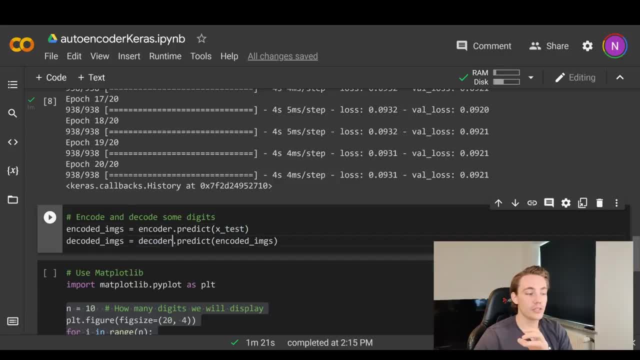 Then we just pass in our test images And then we're also going to decode here again, which will just be where we're predicting on our encoder images, because the results here of our encoder images is actually like our Code vectors. So this is our original input image. 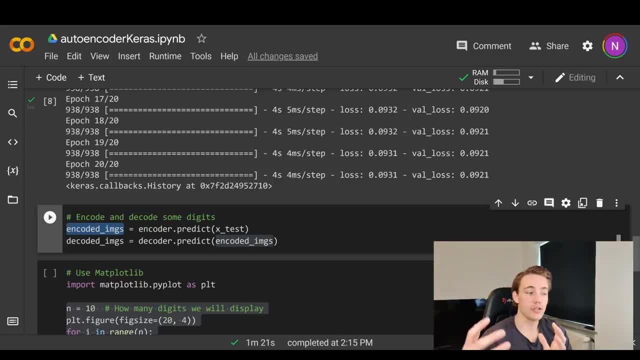 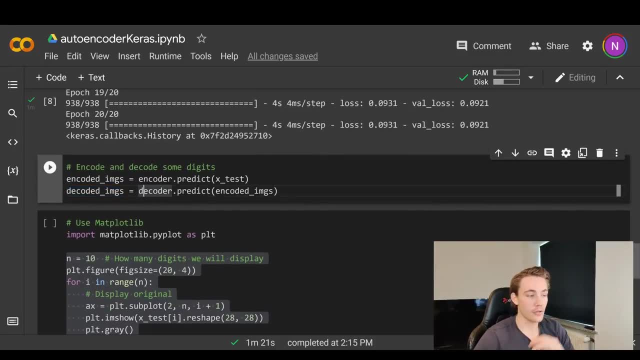 This is our code vector. Then we pass in our code vector and try to decode that again And then we will actually like have our decoder images or our reconstructed images so we can see what is actually like going on. So these images ideally should be exactly the same as these images that we pass in. 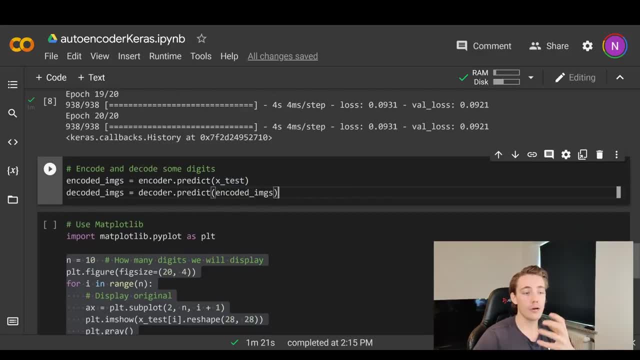 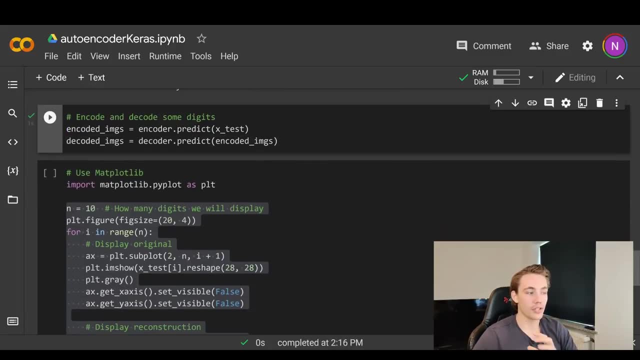 here in the encoder prediction input. But now, as we can see, we get a loss around 9% of those images. but now we're going to run a blog code and we will just do prediction On our encoder and the decoder side. 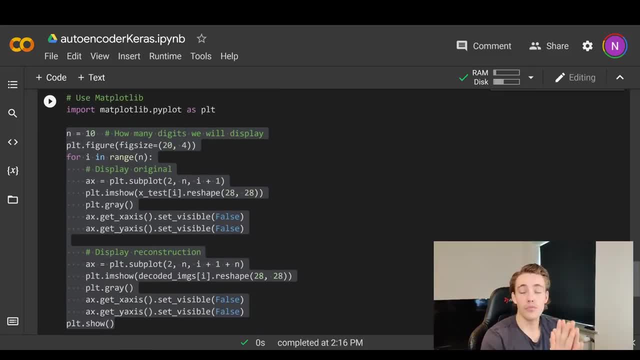 And then down here we're just going to use matplotlib to actually like display both the input image, So like the ground truth image, and also the reconstructed image, So we can see how much loss do we actually get. or like how good is our neural network acts, like to reconstruct our image. 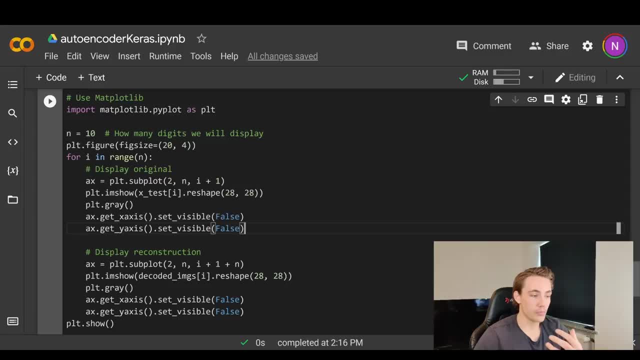 So here we just have a follow running through the number of images that we want to display, and then we just like in show them with matplotlib. So we won't go into details with that, We're just going to run it. blog code. 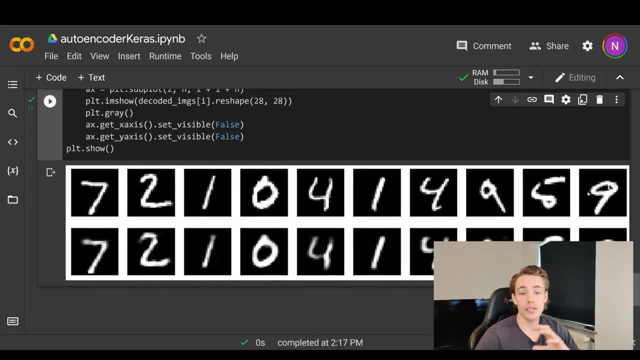 And then we can see down here that the first row here is all the the true labels or, like all our ground true images, and then we pass this through our auto encoder and this will be the reconstructed, reconstructed images from our 32 dimensional code vector. so, as we can see, this is a really nice reconstruction. again, remember, we're only using 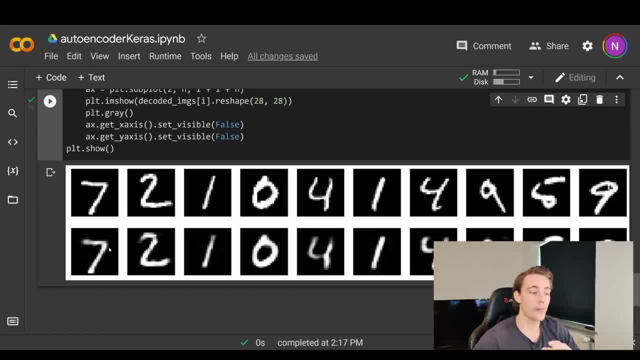 one input layer, one code vector and one one decode layer. so this is a really really simple neural network with not that many neurons. we can see how fast it was to train and also do predictions on later on. it took four seconds for each of the epochs, but training on 60 000 images it took. 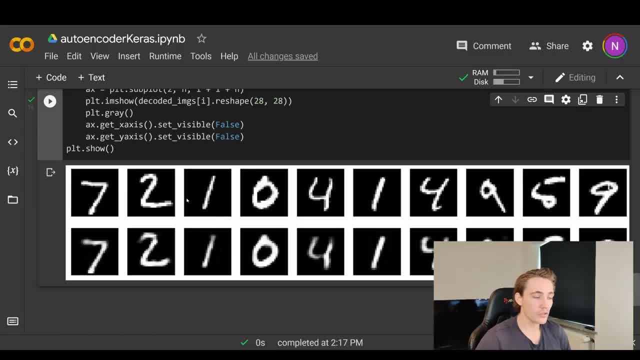 four seconds to train on 60 000 images. it just shows like how simple the model is and how good the results actually are. so we see the seven here is actually reconstructed pretty good. two again really good. one zero four, one four. we can see here with nine we get some more gray areas.